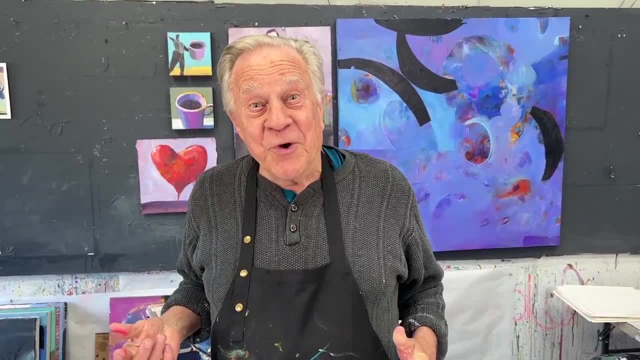 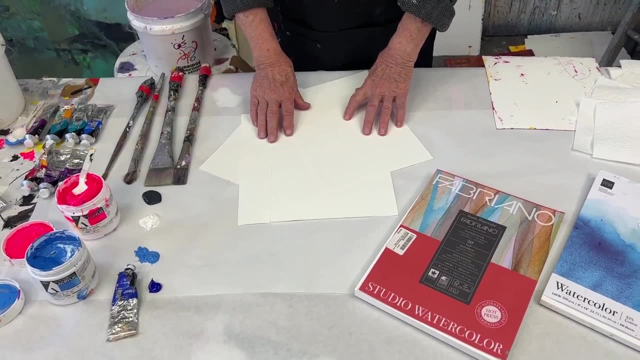 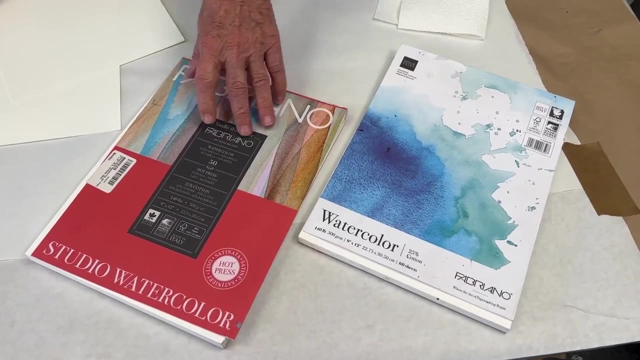 it's a lot more funner to make your own. Here's my table set up just to show you this demo: Big brushes paper. My paper happens to be Fabriano and it happens to be watercolor paper Perfect for handling paper and paint. I'm going to show you how I make my paper. I'm going to show you how I make my 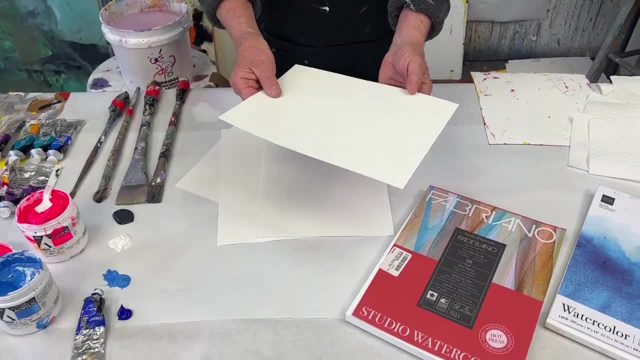 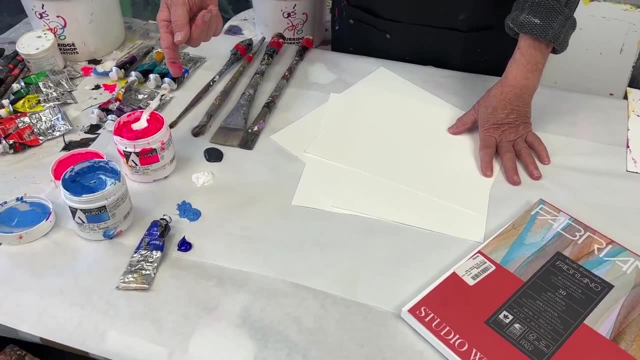 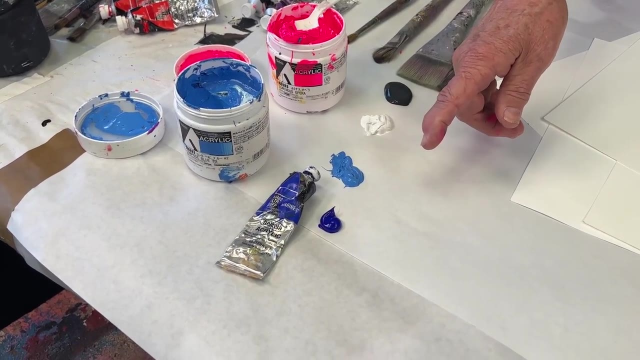 water and paints and anything, and it takes a beating. I really do like Fabriano watercolor paper. Now the paints I'm using will be blue, of course. This will be blue. This is cobalt blue, or I could also use an ultramarine blue. Those two blues are great for mixing the periwinkle color. 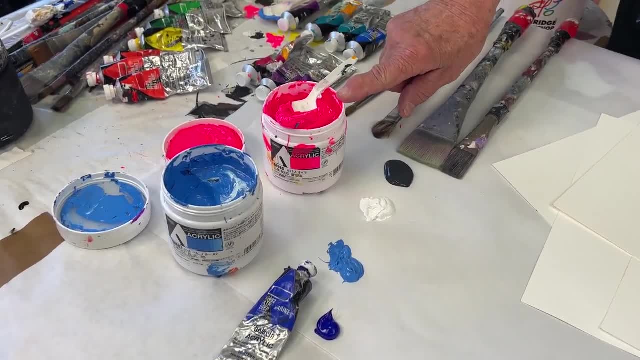 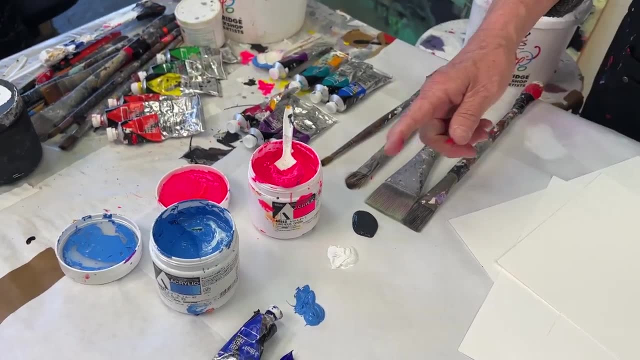 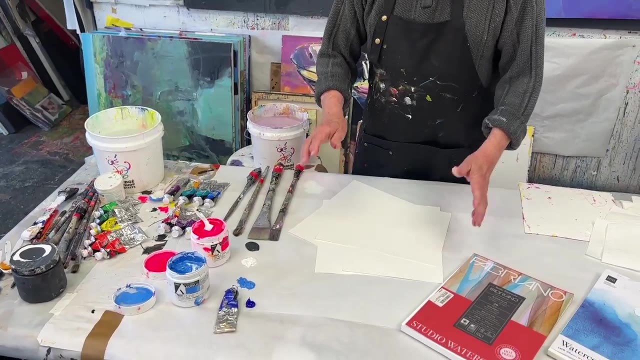 and I have my hot pink. It's that opera from Holbein. There you go: Fluorescence Pink, They call it opera. I love that color, and I do have my white, of course, and my black. So this is just a demo to show you how to mix your own. I'm going to continue on. 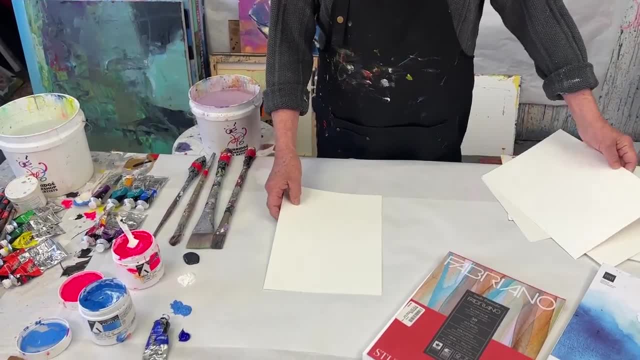 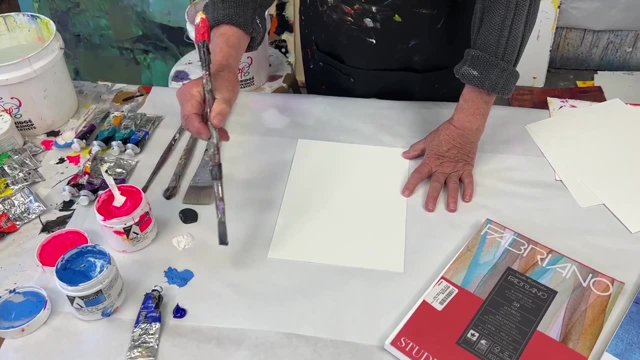 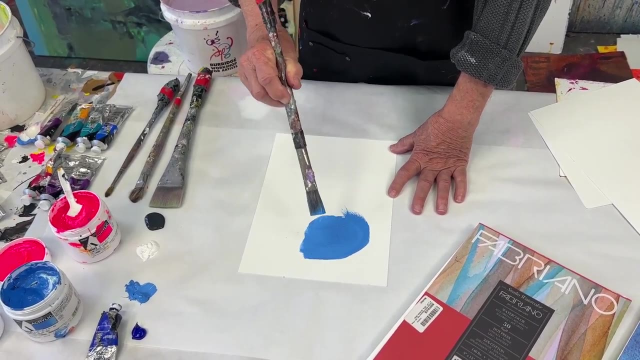 just to show you how I mix it. This is a great fun thing to do in your studio. First thing I'm going to start off with will be a little bit of blue. Lots of water on my brush. Lots of water on my brush. Now here comes the magic color opera. 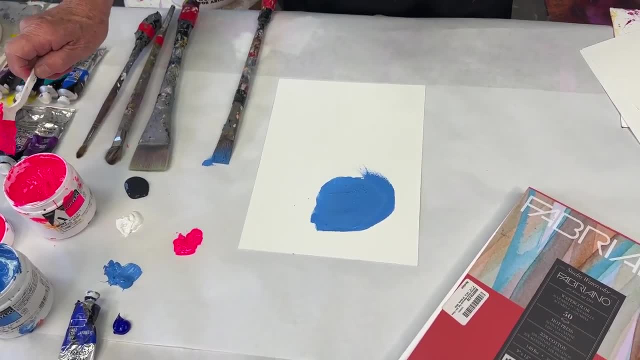 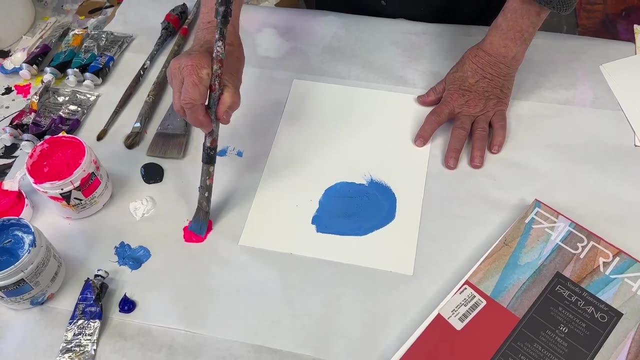 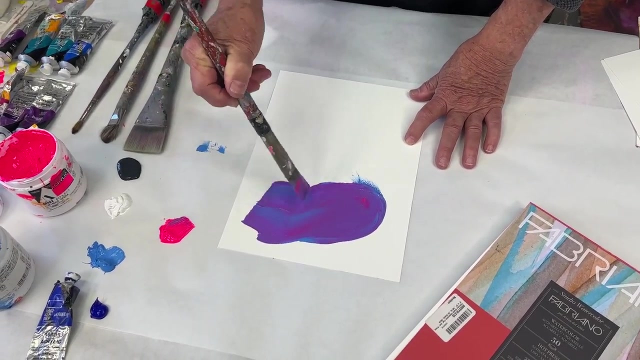 When was the last time you dished out your own color and go whoa right. Well, you're going to do that with this one. Here's the opera, mixing it right into this paint. So it's somewhat on the purple side. I just wanted to let you see. 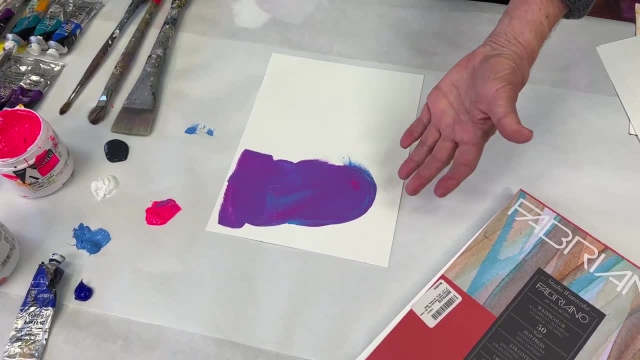 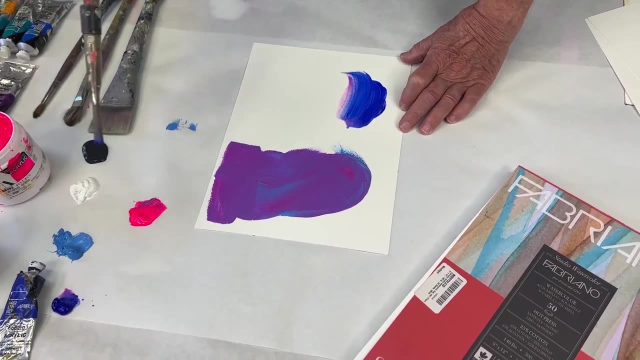 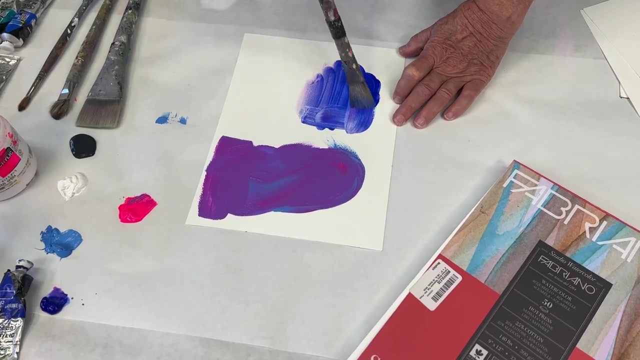 it's going to end up differently. It depends on the color blue that you use. depending on the blue that you use, but here's ultramarine blue. that, by the way, was compost blue, number one from holbein. here's the wonderful color of ultramarine, but wait, wait. 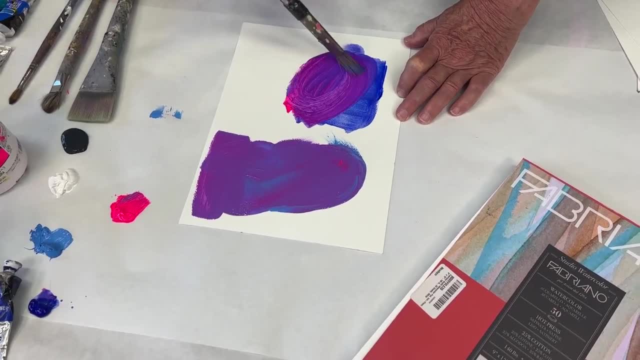 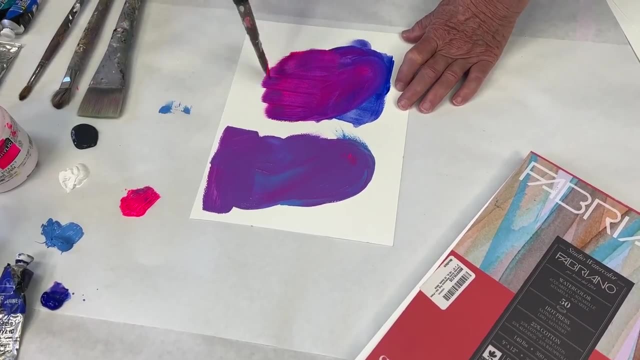 till we start adding this pink to it. here comes your periwinkle, a lot different than that one, and you can adjust it by adding more colors. look at the difference. it's still periwinkle. now, if you wanted to, let's add some white to it. 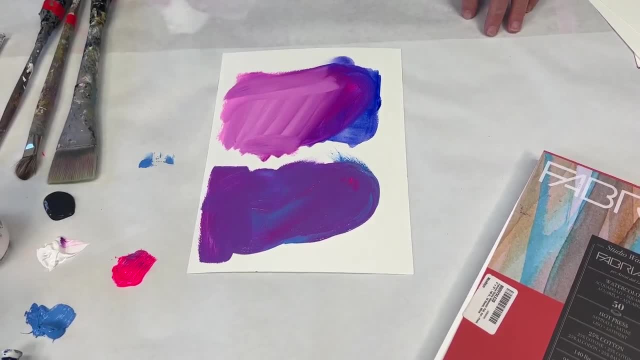 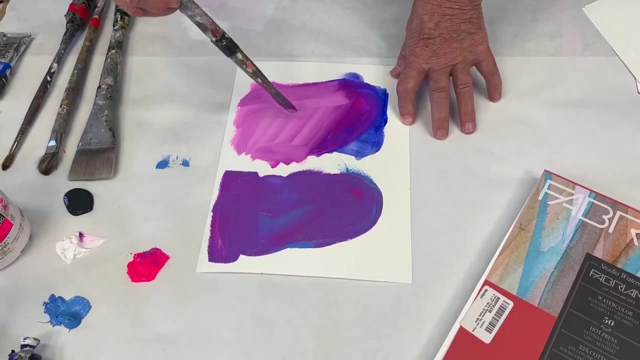 oh jeez, look at all the wonderful colors you can can get, just with blue. and then opera, color, fluorescent opera. there's your periwinkles and it just works all over the place. you can even do here's some black. oh wow, look at that. there you go, there you go. 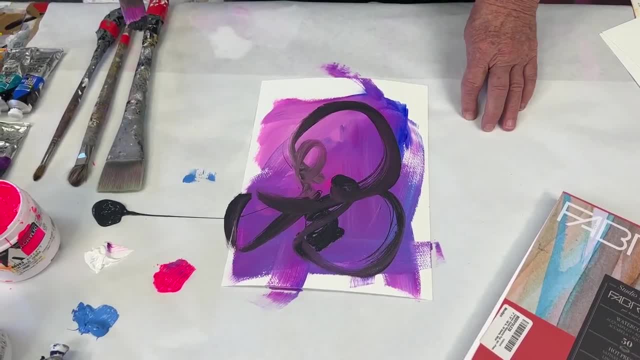 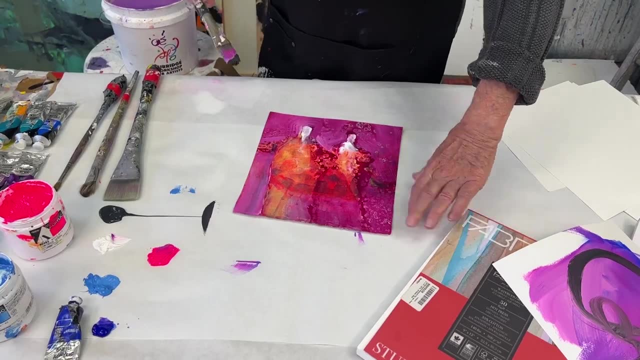 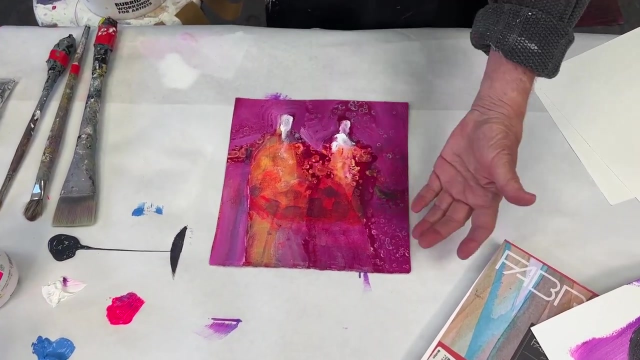 look at the color, how it pops. so let me take an actual painting that i've been working on. here are two figures with a start- at least I have a start- of somewhat periwinkle, but i'm going to keep this simple, keep this short, and i'm going to paint it so you can see. 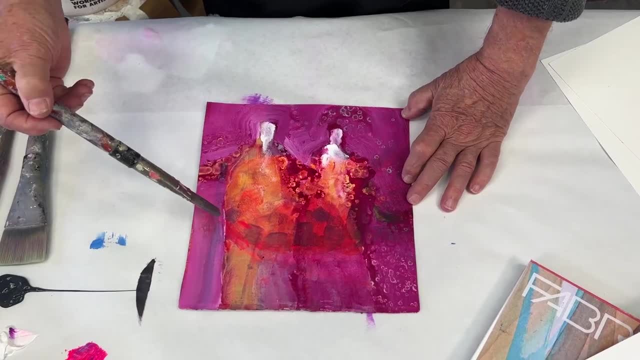 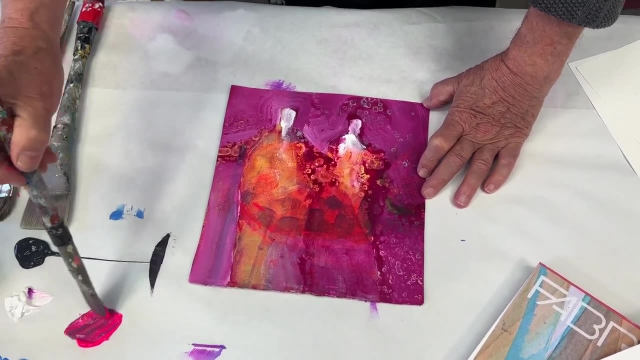 it. so i'm going to go dark up here and lighter down here in the bottom. i've already done the figures. Of course they're very abstract figures. I'm going to mix up my periwinkle, since this is all about periwinkle. 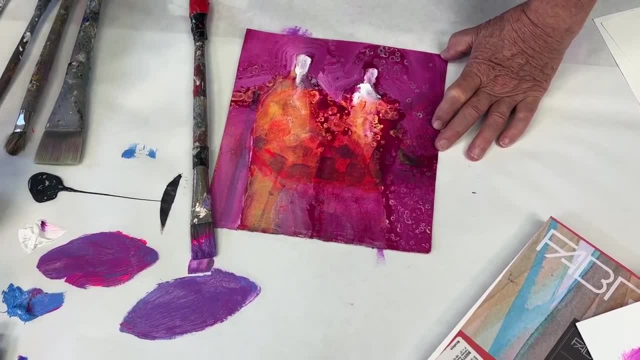 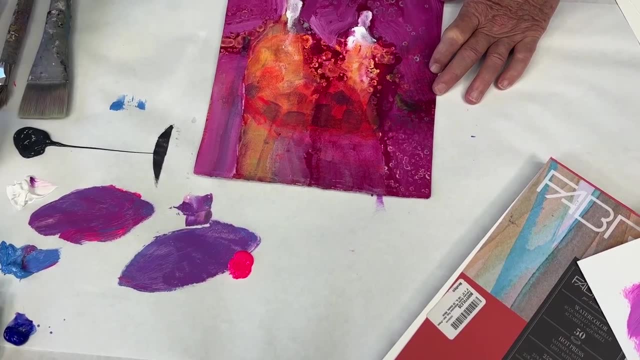 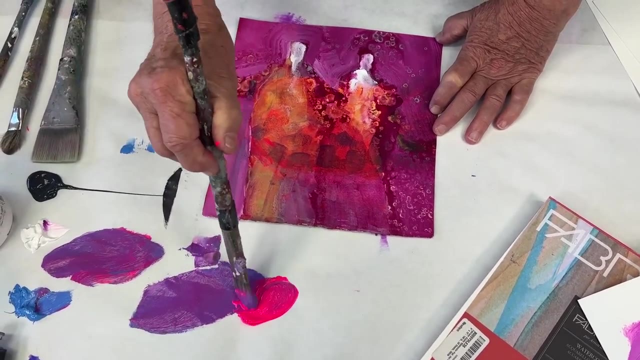 More pink. Some people call this pink, Some people call it opera. Officially it's called Luminous Opera. Remember that name, Luminous Opera? And I get mine at Holbein because the colors are so rich and thick and full of pigment. 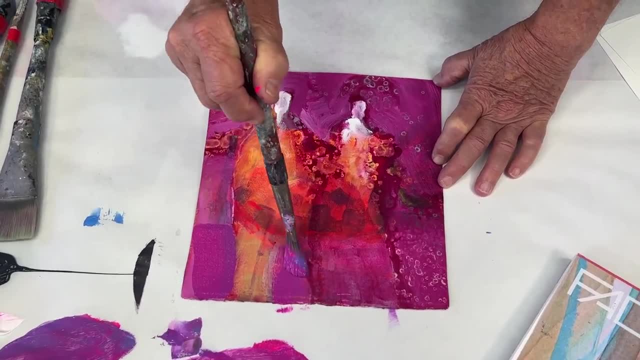 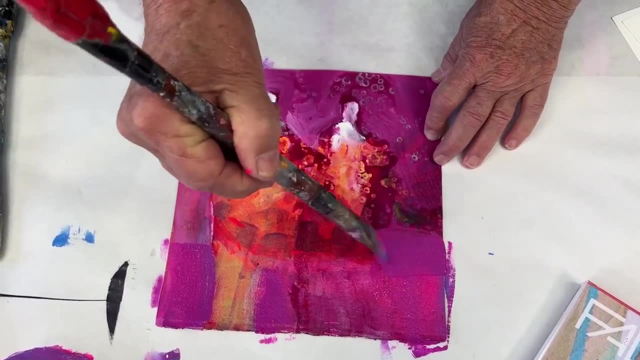 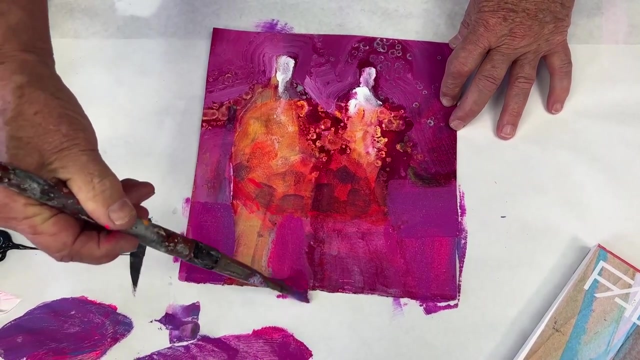 I'm going to do some negative shape painting here, just because it's fun to do. There we go. I'm mixing right into the canvas here. Actually, this is watercolor paper. Yeah, I don't know, I'm going to make it dramatic. 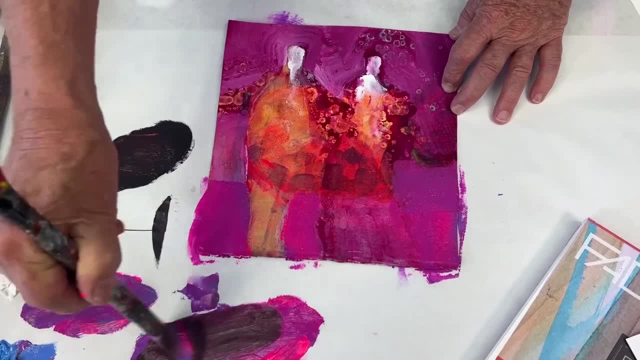 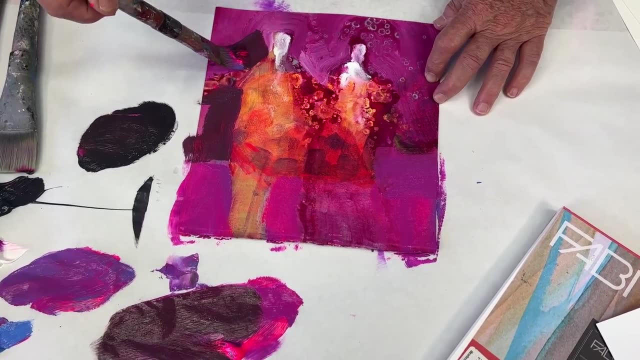 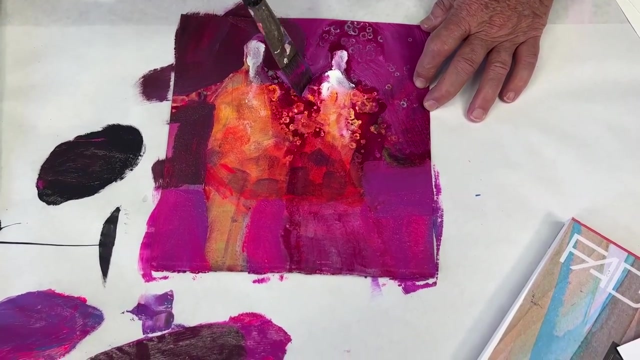 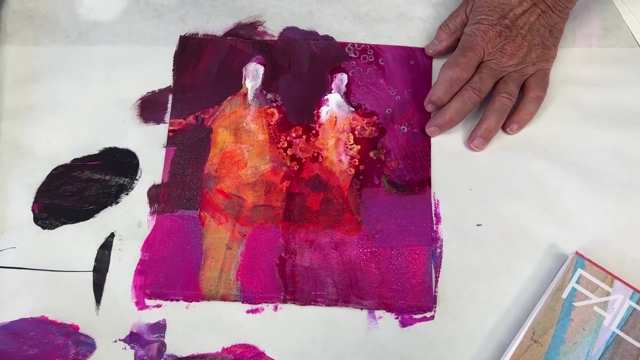 Imagine that He's going to make it dramatic. Imagine that Here we go, Go around the head. There's my head, There's your shoulder, There's your best friends. Nice, big, wide brush. More water on this. I'm going to add evil. 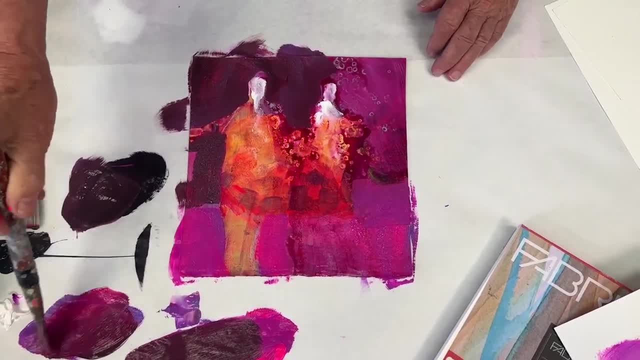 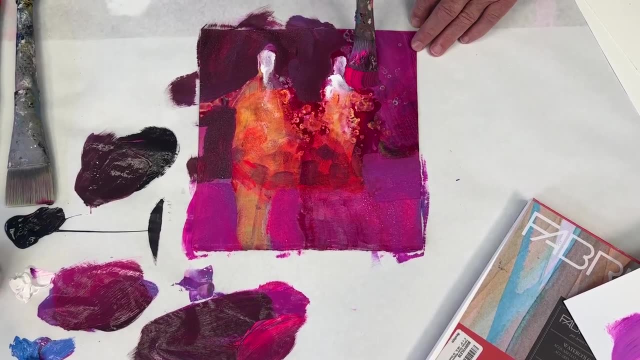 Even more hot pink to this, just so I have some variation, so it's not one solid color. I liked very much to bring in some of the color that's not even mixed into the blue See. it gives it a little bit of a shimmering look to it. 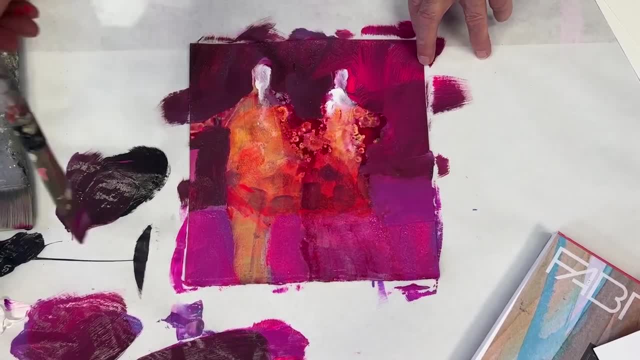 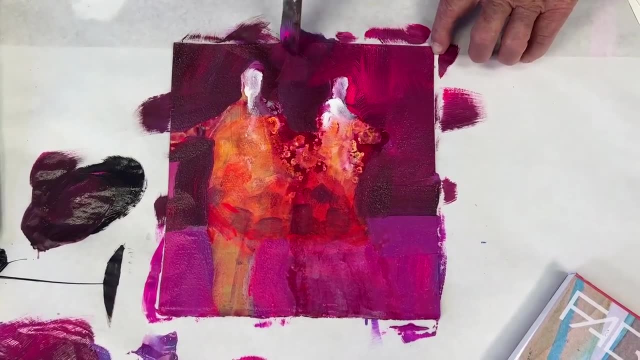 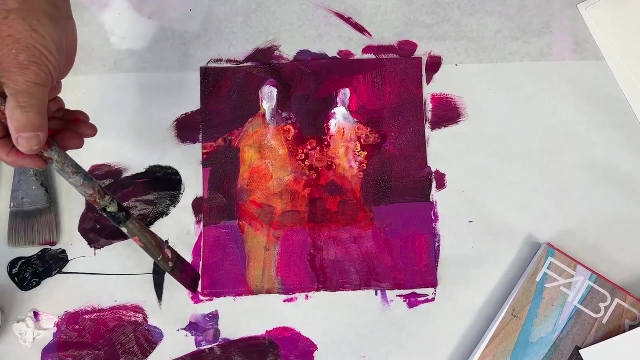 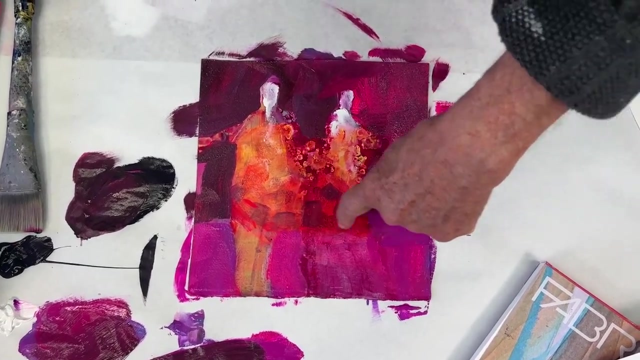 Ah, cool, Whoa, Whoa. Now we have a background So dramatic, almost monochromatic: dark light, two focal points. This is called Friends. Now, if you wanted to clean this up, I happen to like all the variations. 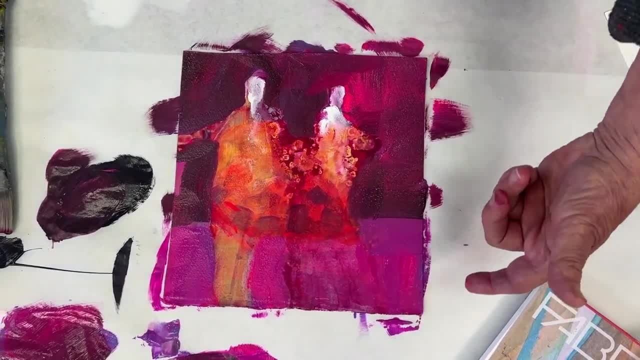 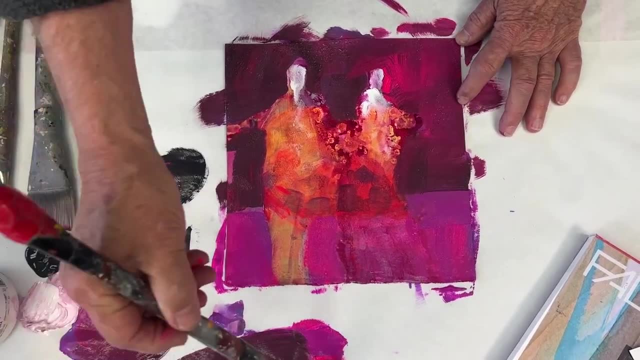 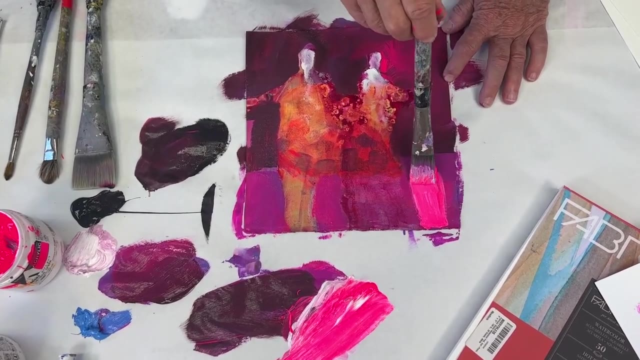 Just to show you in this demo all the different effects you can create with just that one color: the opera. I'm going to add more down here to make it even more dramatic. Look at this: Whoa, Wow, I love the surprises this creates. 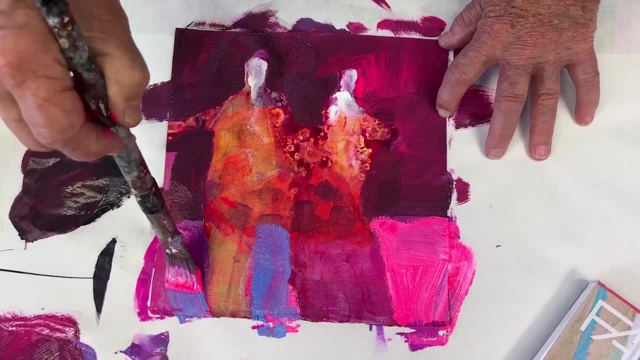 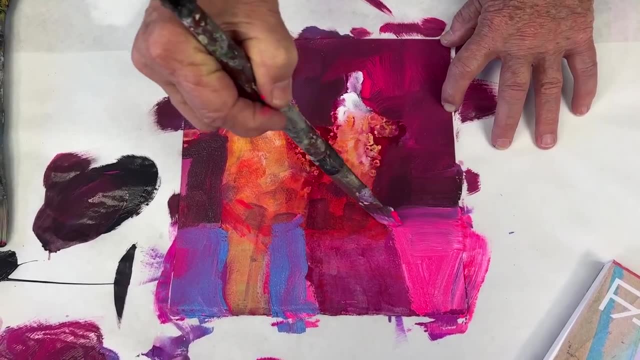 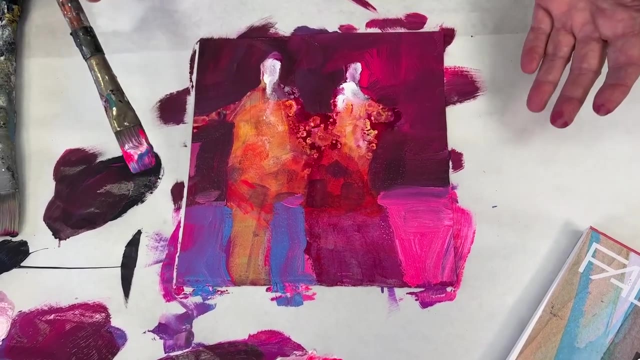 And I'm bringing the blue back into here, Even though it's not mixed into the pink. I happen to like the shimmering effect and the painterly effect of all of this Dark light back and forth. It's very important that you paint all over the painting. 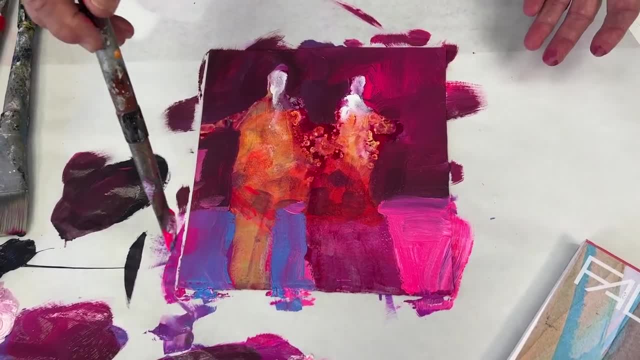 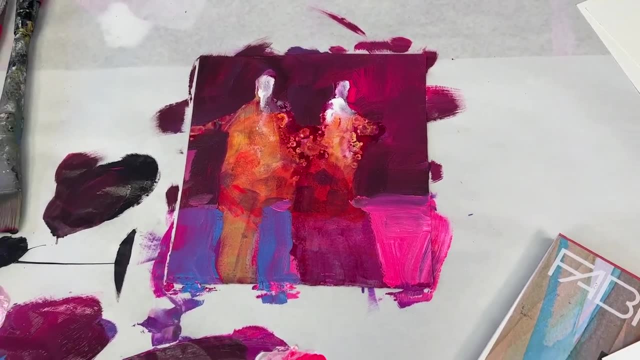 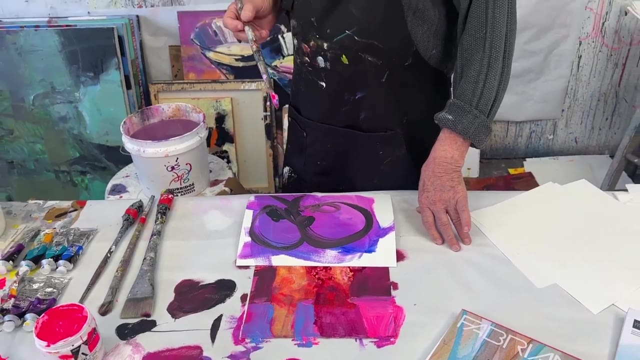 All at one time. Don't stay in one place. you'll just tickle it to death. No way to kill it right. There you go. Well, that's Periwinkle. It's a pretty simple little demo, But let me tell you, play with that luminous opera and you can't go wrong. 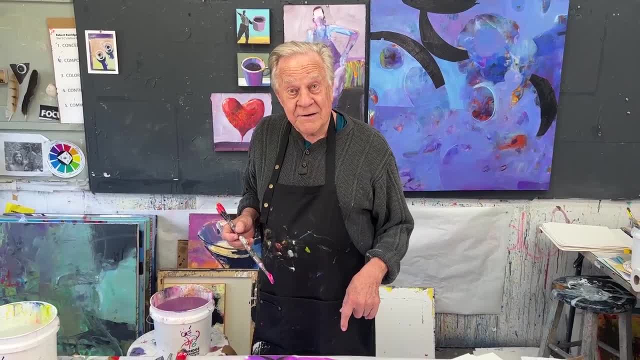 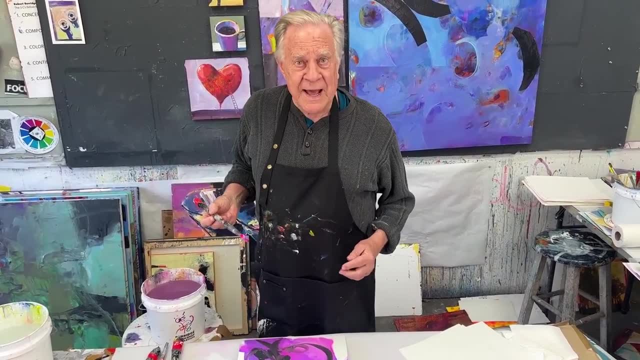 Lots of white. There's even black in here. Yes, I use black. I've heard so many people say you use black. I've heard never use black. I've heard never use black And I always like to say: why say that? 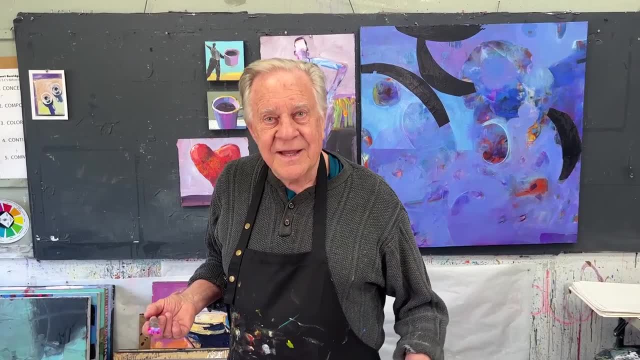 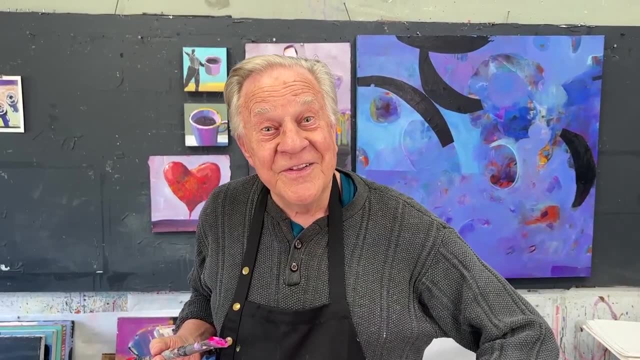 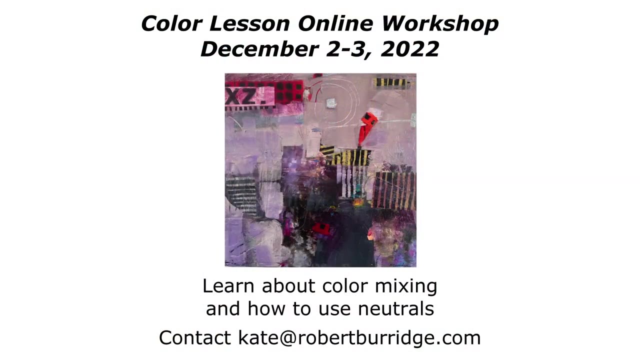 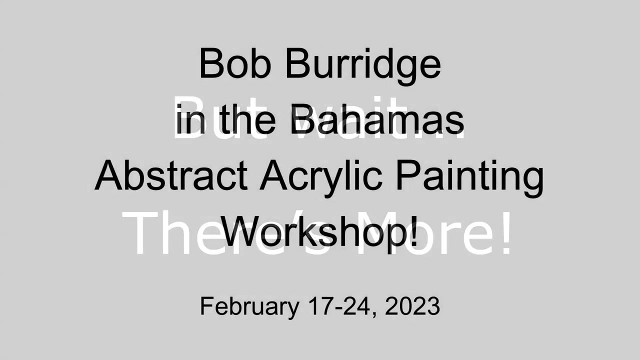 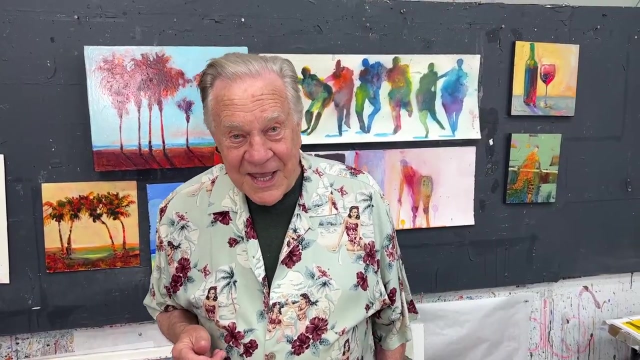 Because they sell it in the art store. So, yes, I use black and white to make my own Periwinkle. Hey, keep your brushes wet. I'll see you on the next Bob Blast, Take care Bye. Hi there, I'm Bob Burrage and we're going to the Bahamas this February. 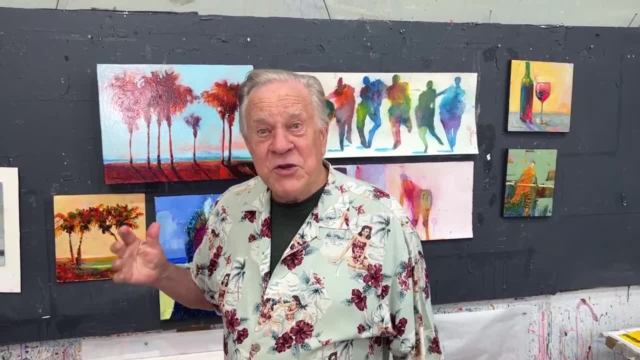 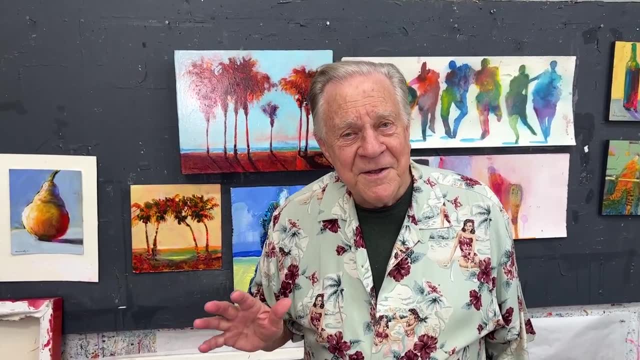 I cannot wait to go there with you. Can you imagine doing a workshop painting by the beach, by the poolside, for five days of painting? I cannot wait because it's most relaxed. I call it a paintcation. Can you imagine painting every day? 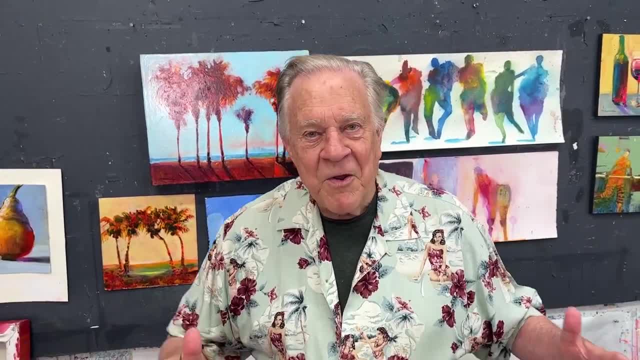 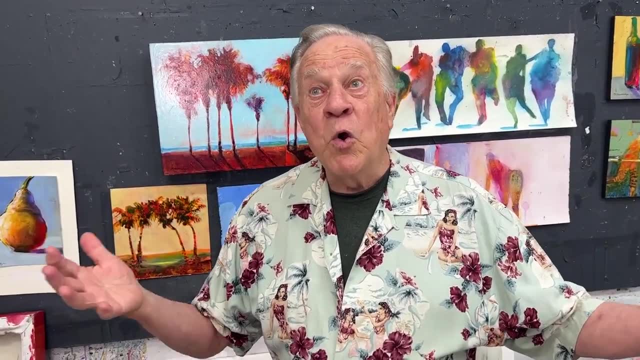 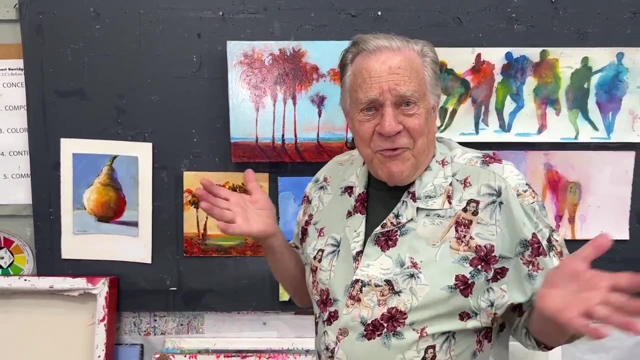 But there's the bar, there's the beach. We're right there, We're relaxed And we're creating wonderful paintings in this incredible Bahama aromas, The florals and the wonderful aromas of the food cooking and the ocean right there, fresh air. 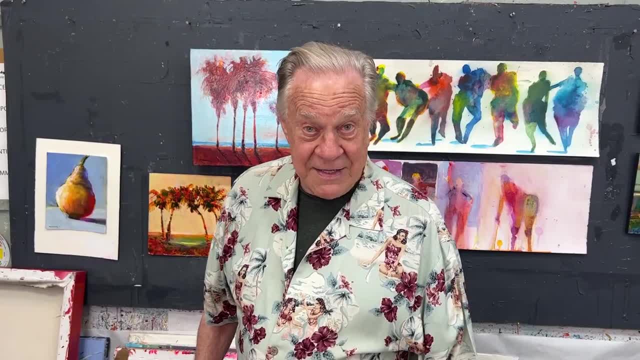 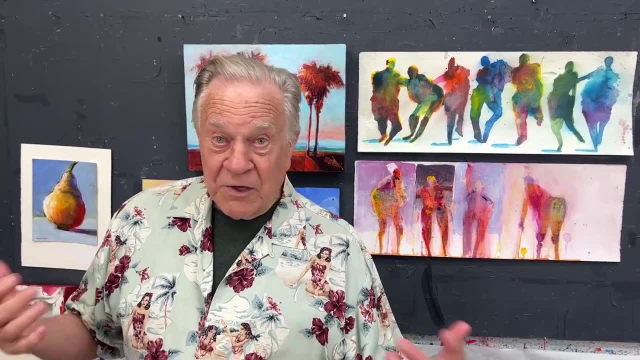 Perfect time of the year to get away right And to have a great time. It's my favorite place. I call it a paintcation. What a great name for it- A paintcation, And we're going to be painting loose.